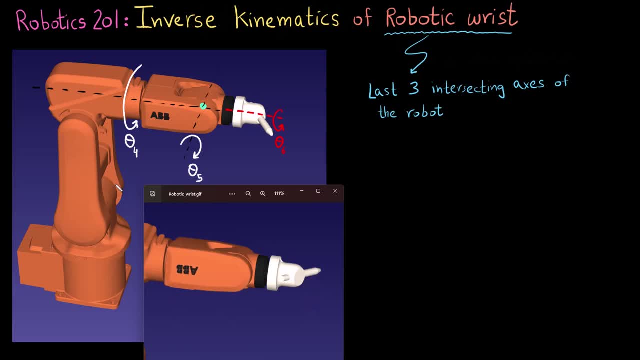 Now I am just changing theta 4 with theta 5 and theta 6 constant, And then I will just change theta 5 and keep the other two thetas being constant. So now I am just changing theta 6, while keeping theta 4 and theta 5 constant. 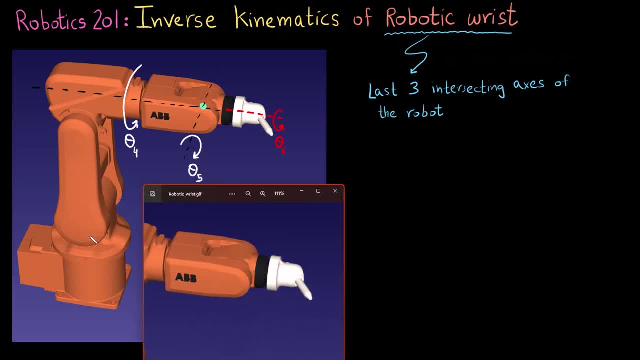 And then I will just change theta 5 and keep the other two thetas being constant. So now I am just changing theta 4 with theta 5 and theta 6 constant, And then I will just change theta 5 and keep the other two thetas being constant. So now I am just changing theta 4 with theta 5 and theta 6 constant, And then I will just change theta 5 and keep the other two thetas being constant, And then I will just change theta 5 and keep the other two thetas being constant. 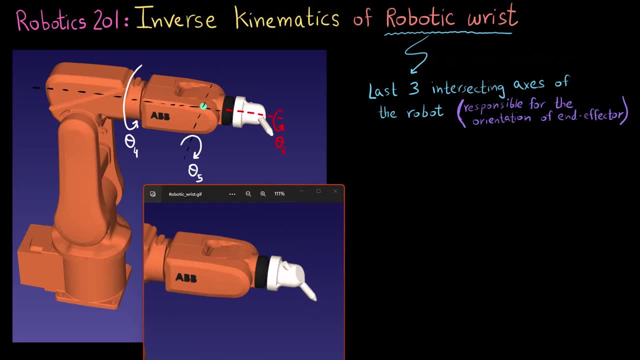 And then I will just change theta 5 and keep the other two thetas being constant. So now the question is: what is inverse kinematics? But before we answer that, we need just a recap of the previous video that the robotic wrist is responsible for just the orientation of the end effector. 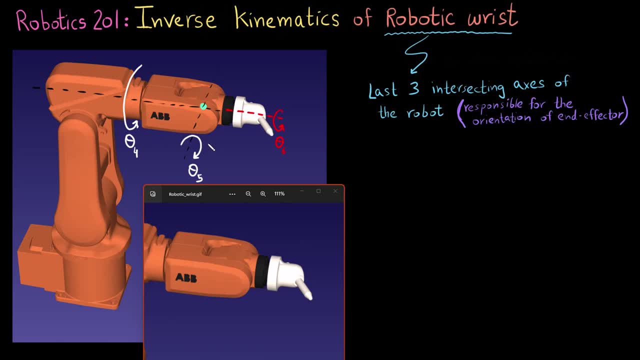 So the the last three intersecting axes. these do not define where the end effector is going to be, as in the position. they only define the orientation of the end effector. So just keep that in mind. And, And now, what is the inverse kinematics of robotic wrist? 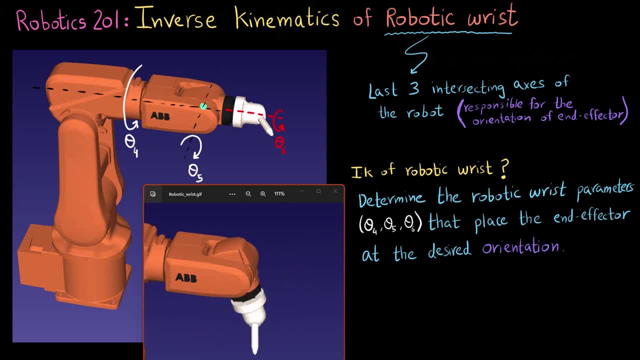 It is basically to determine the wrist parameters, which in this case are my theta 4, theta 5 and theta 6, that place the end effector at the desired orientation. Again, notice the word orientation, because we are talking about the robotic wrist, which is the last three axes, and these are only responsible for the orientation. 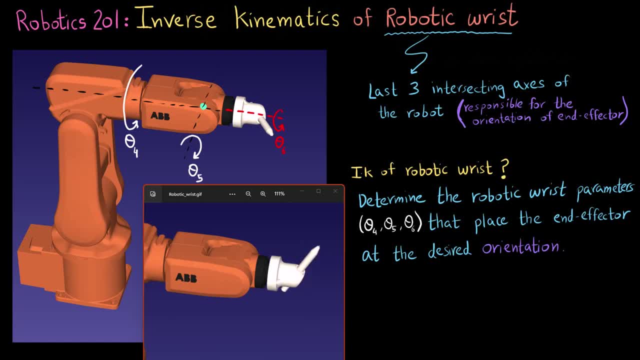 and for this robot, the first three axes of rotation would be responsible for the position and the three are going to be responsible for the orientation. similarly, if it was, let's say, a seven degree of freedom robot, so the last three x's are always going to be responsible for the. 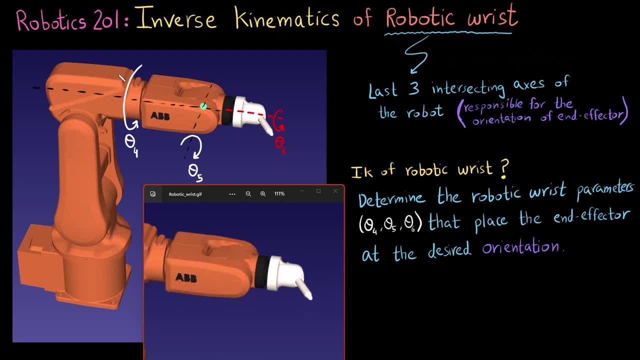 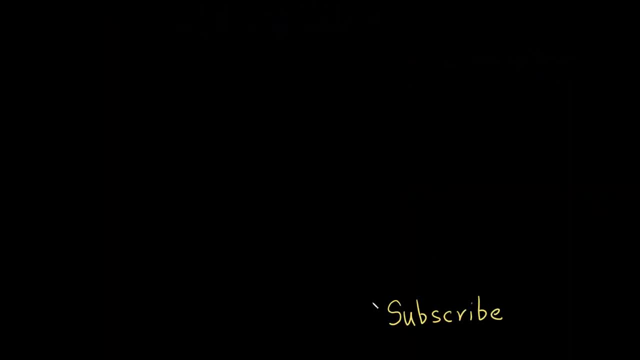 orientation, and all the x's before the last three are going to be responsible for the position. let me keep this video short and in the next video we are going to do a numerical example as to how do we actually do the inverse kinematics of a robotic race numerically. 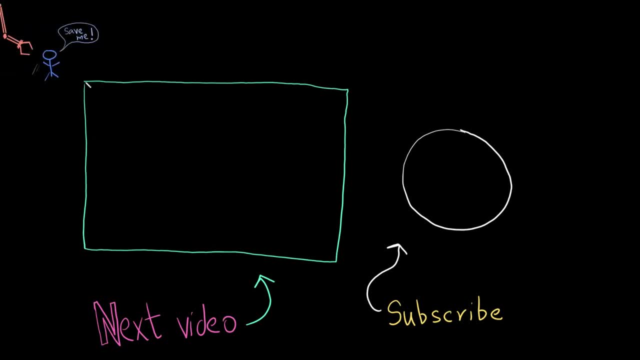 and how do we find the solutions and what do those solutions represent. so see you in the next video. thank you for watching.